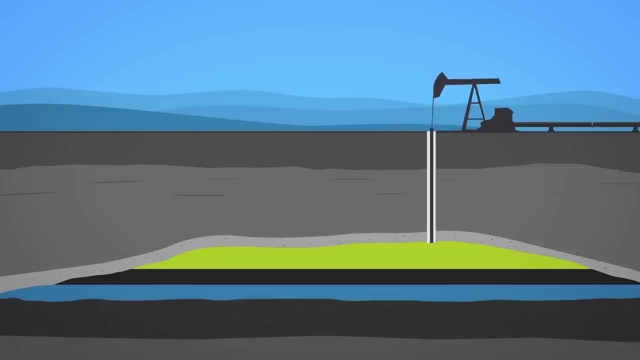 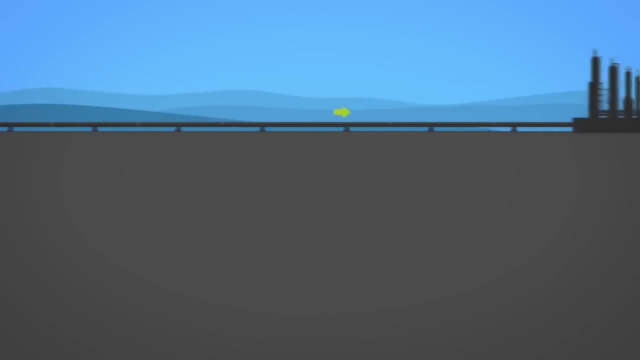 sometimes extracted alongside oil. This type of natural gas is called associated gas. In the past, associated gas was commonly flared or burned as a waste product, but in most places today it is captured and used. Once extracted, natural gas is sent through small pipelines called gathering. 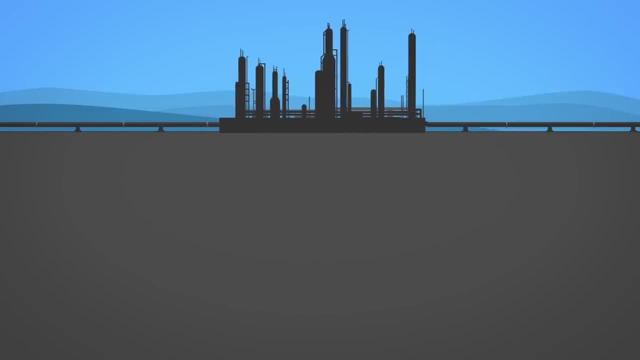 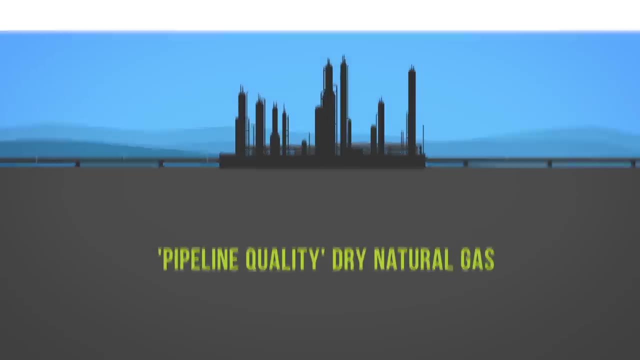 lines to processing plants which separate the various hydrocarbons and fluids from the pure natural gas to produce what is known as pipeline quality dry natural gas. before it can be transported, Processing involves four main steps to remove the various impurities: Oil and condensate removal. 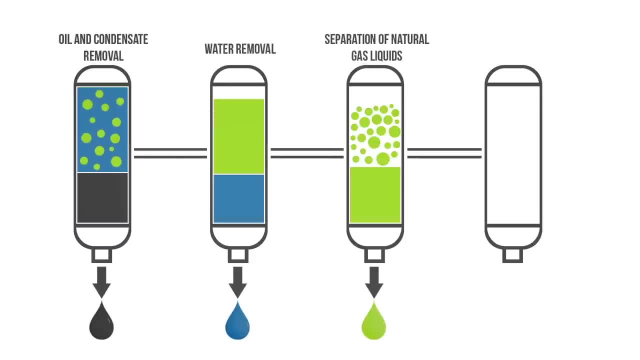 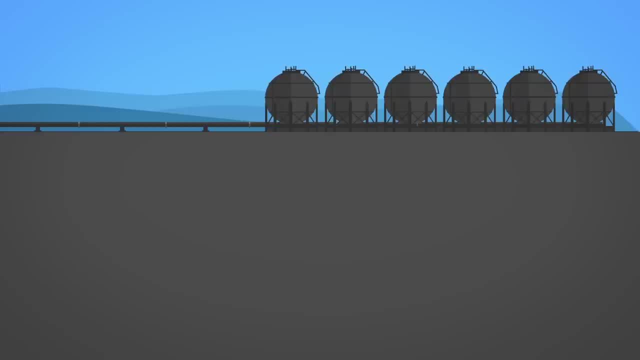 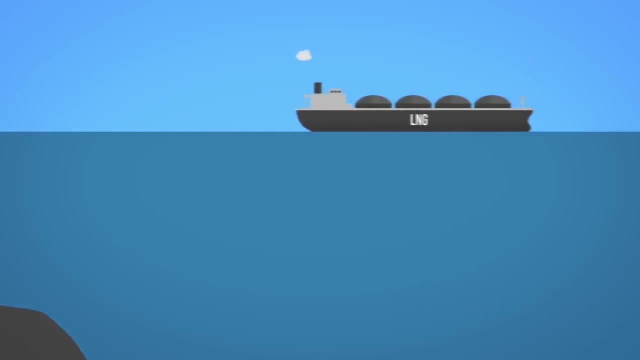 water removal, separation of natural gas liquids, sulfur and carbon dioxide removal. Gas is then transported through pipelines called feeders, to distribution centers or is stored in underground reservoirs for later use. In some cases, gas is liquefied for shipping in large tankers across oceans. This type of gas is called liquefied natural gas or LNG Natural gas. 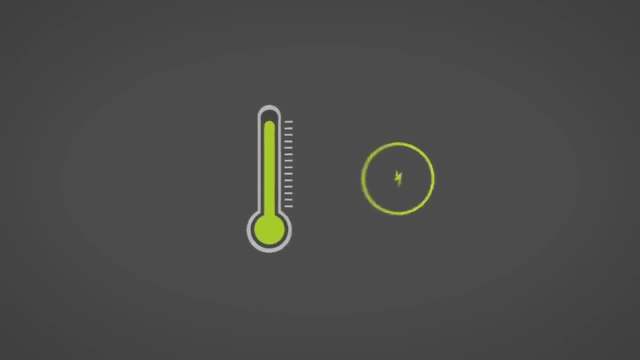 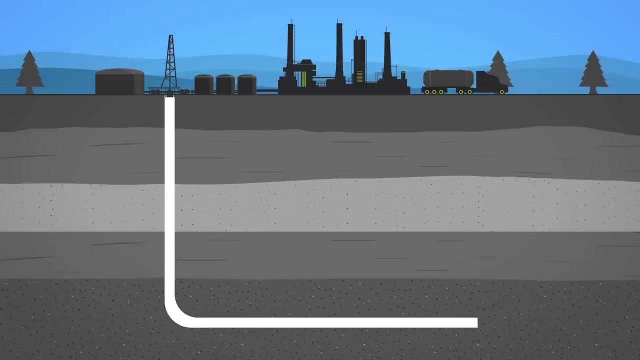 is mostly used for domestic or industrial heating and to generate electricity. It could also be compressed and used to fuel vehicles and as a feedstock for fertilizers, hydrogen fuel cells and other chemical processes. Natural gas development, especially in the United States, has increased as a result of technological advances in horizontal drilling and hydraulic 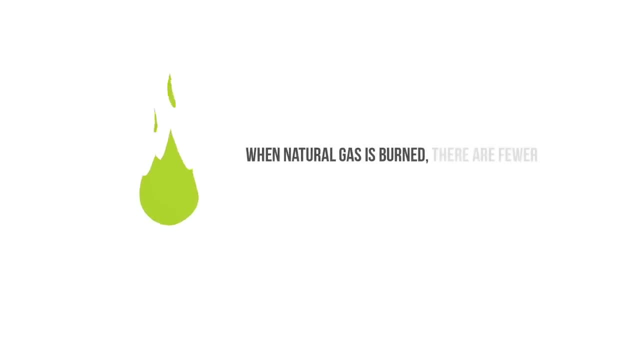 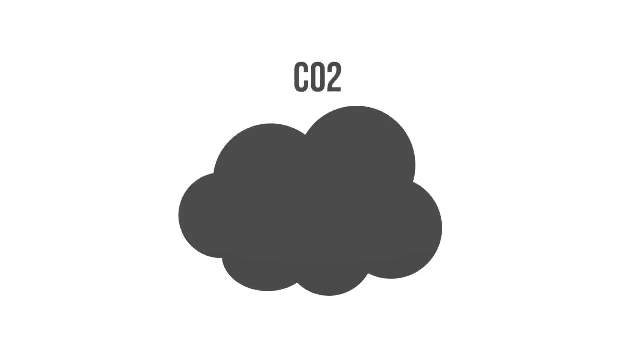 fracturing. When natural gas is burned, there are fewer greenhouse gas emissions and air pollutants when compared to other fossil fuels. In fact, when used to produce electricity, natural gas emits approximately half the carbon emissions of coal. Despite fewer emissions, natural gas is still a source of CO2.. In addition, 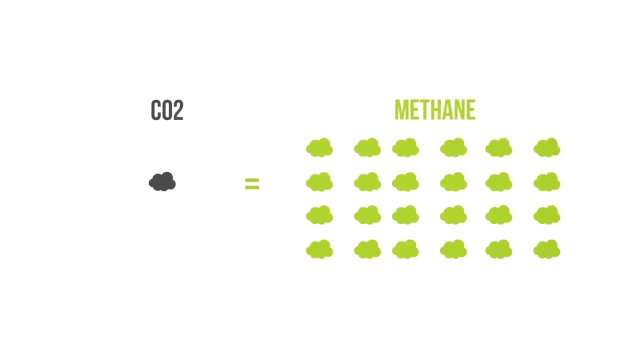 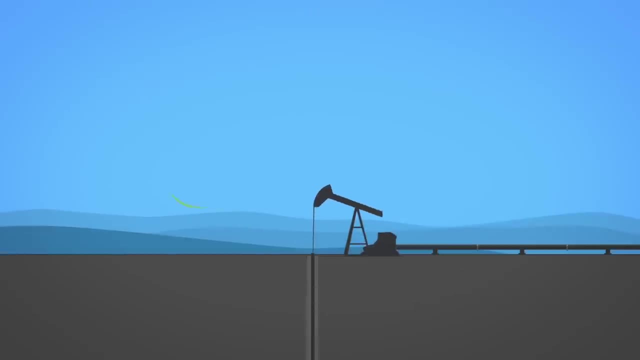 methane is a potent greenhouse gas, itself having nearly 24 times the impact of CO2.. During the extraction and transportation process, natural gas can escape into the atmosphere and contribute to climate change. Natural gas leaks are also dangerous to nearby communities because it is a colorless, odorless, highly toxic and highly explosive gas. That's natural gas. 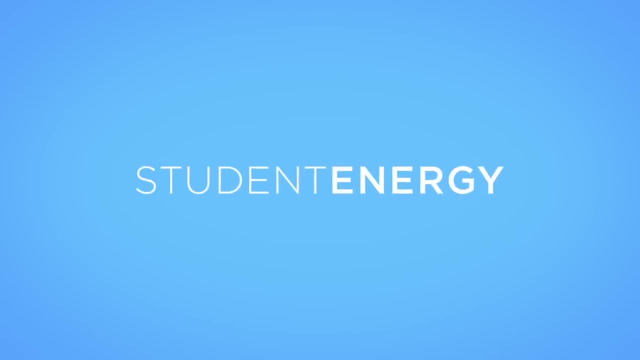 When it becomes harmful to the environment, many people will become vulnerable to it. For more information and information on natural gas and the potential effects of natural gas, go to the linked links in the video description.